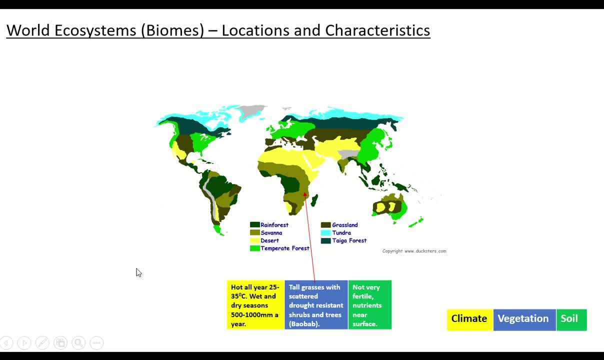 nutrients are found near the surface. So the next biome is the boreal forest or the taiga, and this is where you'd find quite warm summers, between 16 and 30 degrees celsius, but the winters are incredibly cold, with sort of very frozen soil. there. They don't have much in the way of 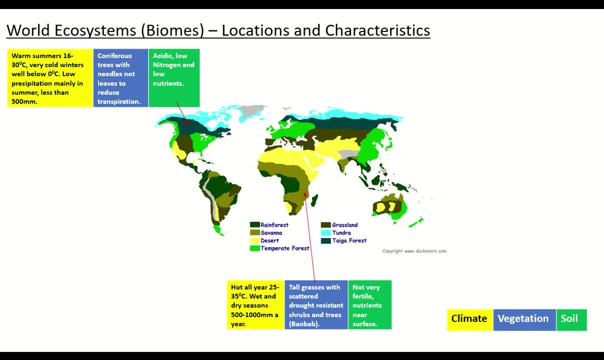 precipitation, mainly in the summer, and it tends to be less than 500 millimetres. In terms of the vegetation you'd find there, it's largely coniferous trees, so think Christmas trees. they've got needles rather than leaves, and that means that the less water they've got. 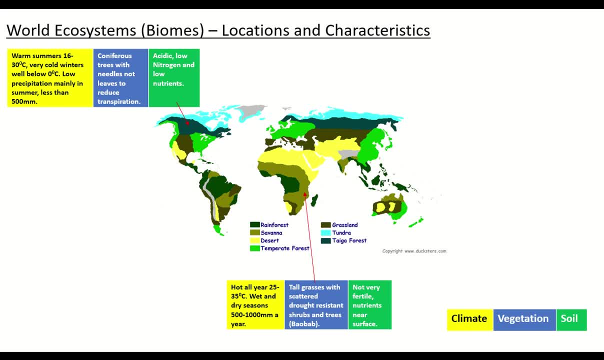 it doesn't matter quite so much because they're not losing so much of it. The soils themselves are quite acidic, low in nitrogen, and they do not have many nutrients. So the next is the grasslands, or the temperate grasslands, and they have hot summers, a bit like. 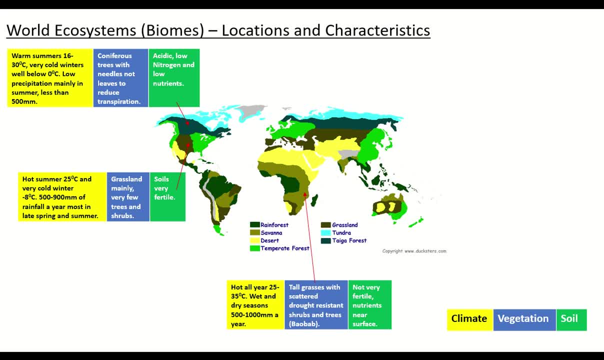 the boreal forests of 25 degrees or so, but the winters are incredibly cold: minus eight degrees. on average, 500 to 900 millimetres of rainfall over the course of a year, but most of it is in late spring and summer. Again, like the savannah, it's largely grassland, very few trees and shrubs. 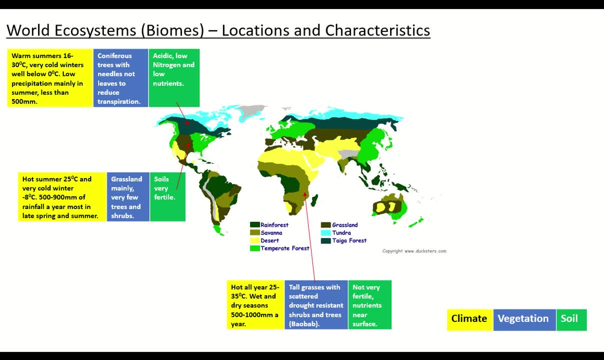 grow there and the soils, unlike the savannah, are quite fertile. So the next one is the tropical rainforests. Now we're going to go into these in more depth later on in this topic. So tropical rainforests have the most consistent and best conditions for. 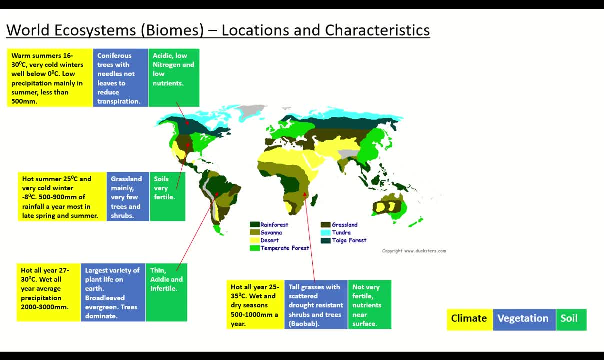 plant life and hence why there there's so much plant life and wildlife that actually lives there. So they're hot all year- 27 to 30 degrees celsius- and they're wet all year as well. The average rainfall is between two and three thousand millimetres. They are the largest variety of plant. 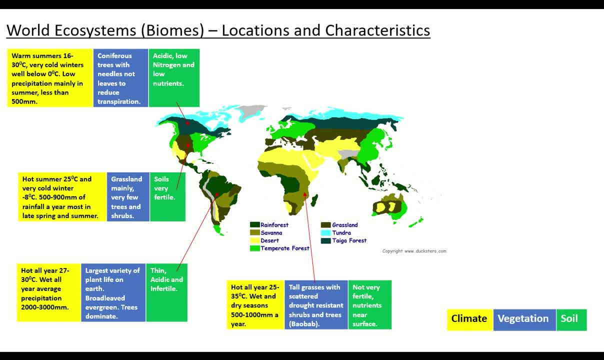 life and animal life on earth. They are broadleaf- sorry, evergreen- trees. They are very rich in plants, mainly trees, and, like I say, lots of wildlife that associates with those habitats. The soils, quite surprisingly, are thin and acidic and largely infertile, but that's mainly because 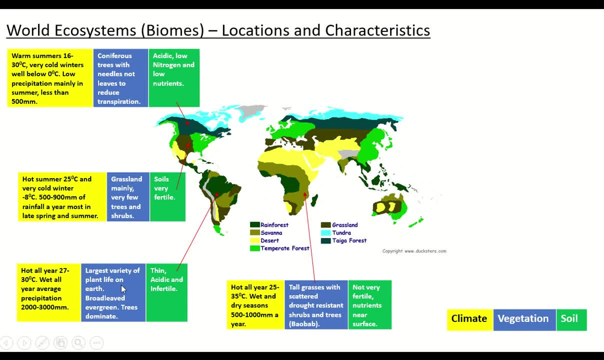 most of the nutrients are actually locked up in the plant life that exists there. So the next one is the deserts, and now these are very hot all year round, very similar to the tropical rainforests, largely above 30 degrees celsius. They do get incredibly cold at night. 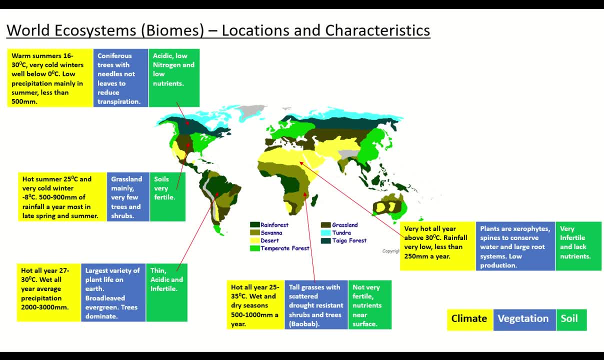 though, because there's no rain, So they're very hot all year round and they're very wet all year round. There's no cloud cover and the rainfall is very, very low and less than 250 millimetres a year. Now, because of that lack of rainfall, it does mean that most plants that you get there- and there's 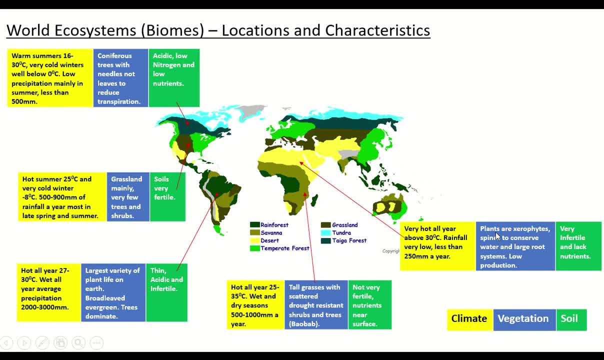 not many of them are what we call xerophytes, and they're plants that can rely on on very little moisture and they tend to have things like spines to conserve their water and reduce transpiration, very much like the conifer trees over here, and they've got large root systems and like, say, low. 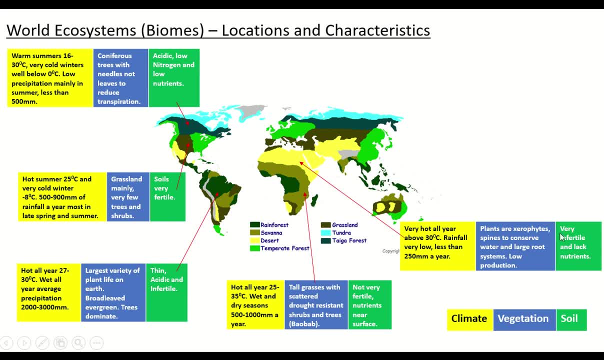 production means there's just a little bit of moisture in there, So they're very hot all year round. The soils themselves, essentially, are sand, so they're very infertile, they lack nutrients and not much organic material goes into them. The next ones are the ones that we'll be familiar with. 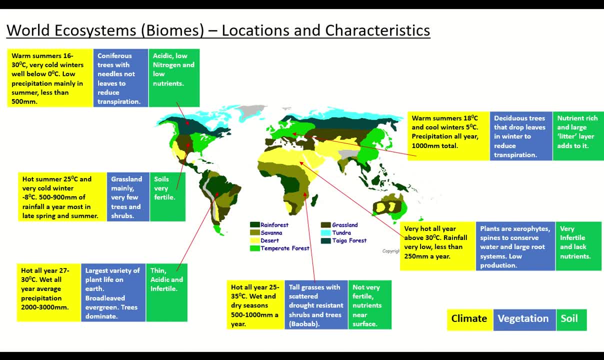 and again, like the rainforests- we'll go into more detail for these- These are the temperate forests or the deciduous forests, So these are the ones we associate with the United Kingdom. We tend to have warmer summers- up to 18 degrees- and cooler winters of maybe five degrees celsius. 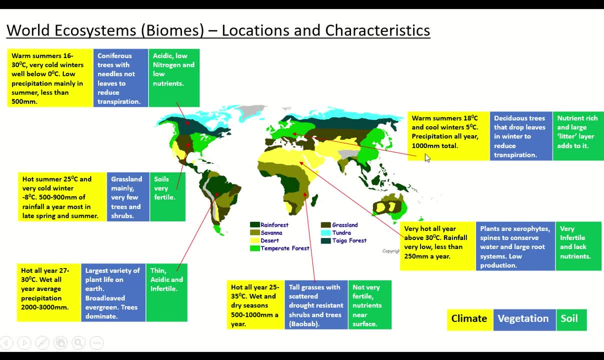 and we do get year-round precipitation, around a thousand millimetres in total on average. The trees we'd find there are deciduous trees, so they'll drop their leaves in winter when there's less moisture available because it's frozen, and that will help reduce transpiration. 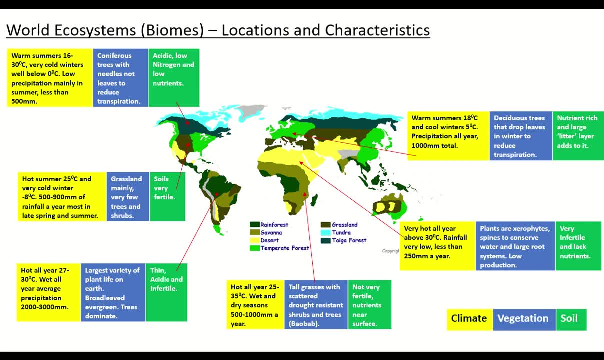 And the nutrients in the soils are incredibly large in the litter layer and that gets decomposed into the soil, so the soils are quite fertile and quite rich. And then, lastly, we've got the tundra region. Now those are the regions you'd find in the north, northern part of the world and the very south. 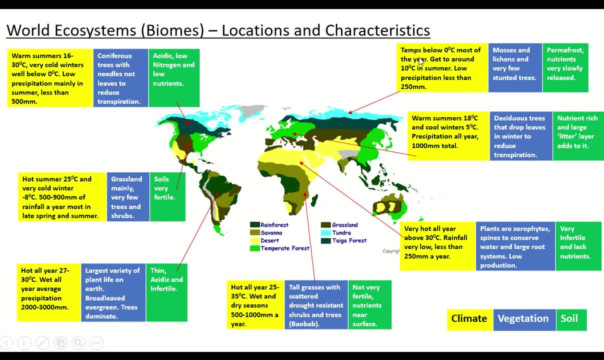 southern part, which is on this map. They tend to be very, very cold, so temperatures are basically below zero degrees most of the year round. They tend they can get up to sort of 10 degrees in summer, but not always. They have very little rainfall, very much like deserts, and that's why sometimes 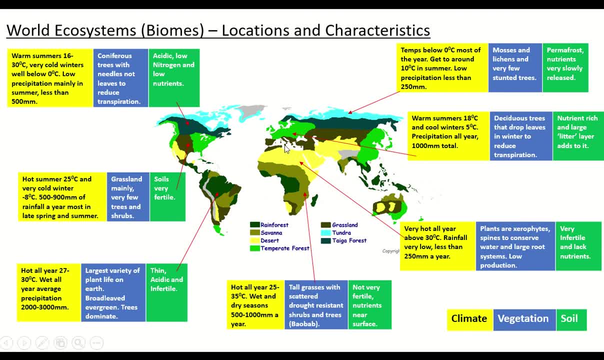 they're called cold deserts- less than 250 millimetres, and again it's largely because air is sinking at these areas. So the sort of plants that can survive these conditions are mosses and lichens and very, very sort of small stunted trees of the hardiest sort of variety. 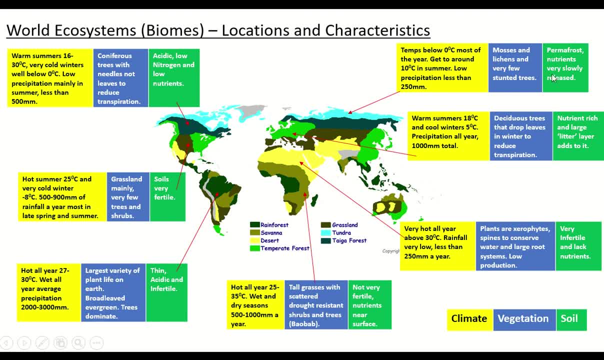 And mostly that's because it's really hard to take root because there's a permafrost and that means the soil is permanently frozen. Nutrients are very slowly released. so any of the trees that grow- they can be very, very small trees of a few feet and have been growing there for years and years- 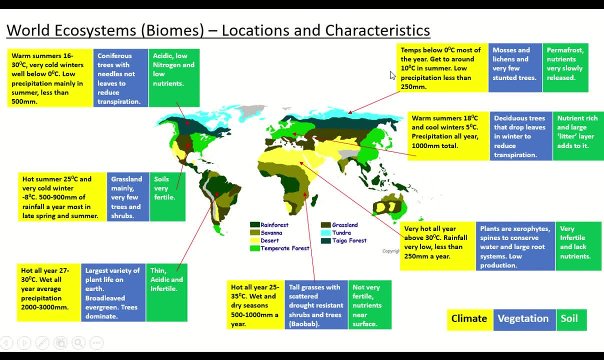 and years, because the nutrients are so slowly released only in a very short summer period and very little sunlight as well. So that summarises really all the sort of seven major world biomes. with regards to their temperatures, the type of vegetation you'd find there and their soil type, It's very likely. 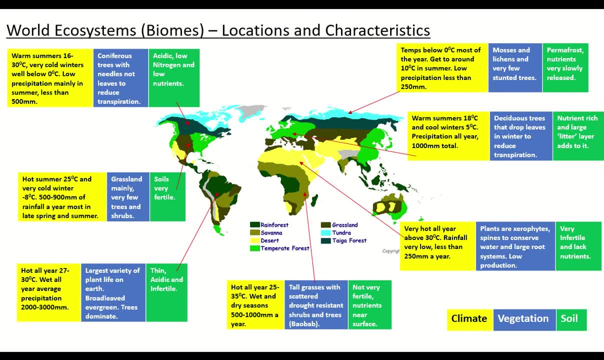 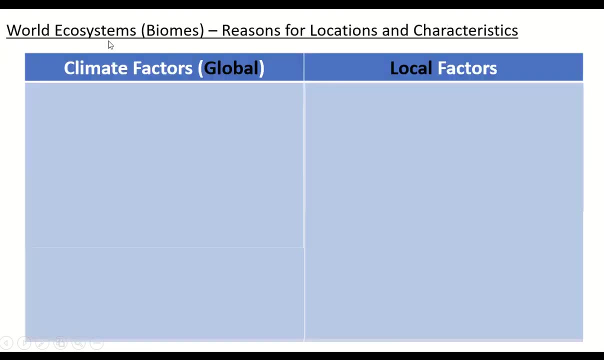 you'll get a question or a small low stakes question about some of these, and so just be aware of where you might find them and the kind of countries that you'd expect to find these kind of biomes in globally. Okay, so another thing that we've got to cover with regards to biomes is the 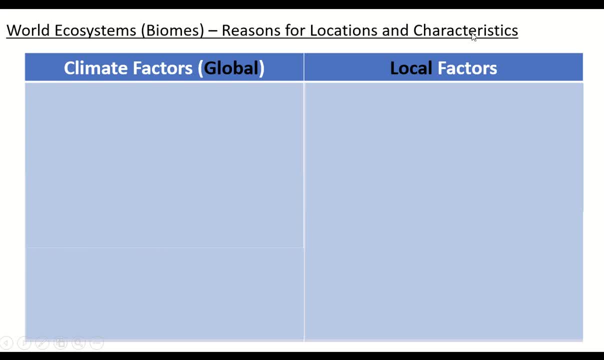 climate. So the climate is a very important factor in the climate research and the reason why they are located where they are located and the reason for their characteristics. So this ties in quite nicely with the other topics from paper one, specifically the weather hazards and climate. 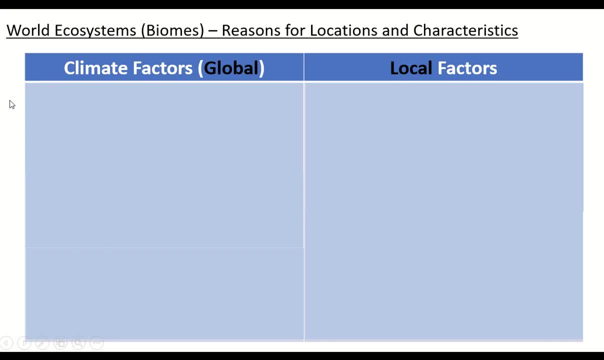 change topic. So, looking at climate factors, these are global reasons why you'd find the tundra where you find the tundra and the rainforest where you find the rainforest. and again think back to the weather hazards and climate change topic. Temperature is one factor, So the further north or 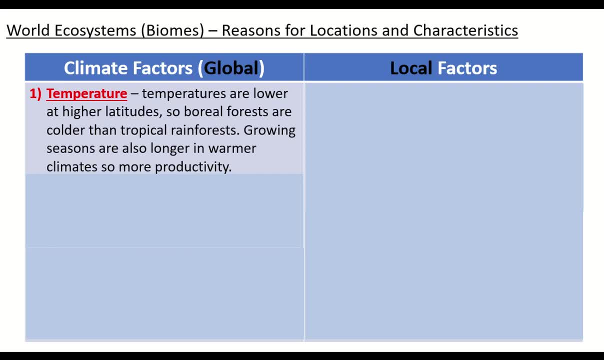 lower the temperatures get, so temperatures are lower at higher latitudes. Boreal forests which are near the north pole are far, far colder than tropical rainforests, for example. It also means that the growing seasons are shorter if you are further north or south, so the longer warmer. 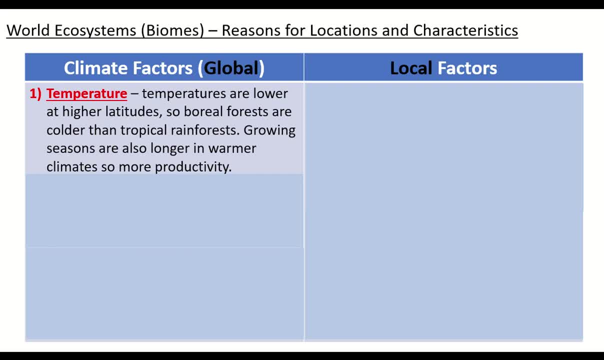 climates near the equator have very much more vegetation because they've got more sunlight and they've got better conditions to grow that. So that's one of the reasons that you'd find the rainforest where you find the rainforests and the tundra where you find the tundra. 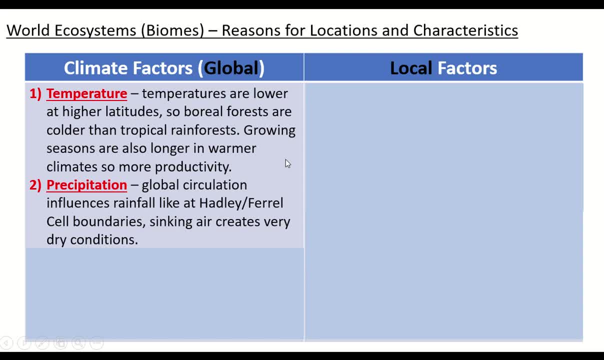 The second climate factor is precipitation. So again, this is why climate is important. Now this ties back into global circulation cells, so Hadley cells which rise at the equator, creating all that rainfall as the air rises, and feral cell boundaries as well. and then you've got your. 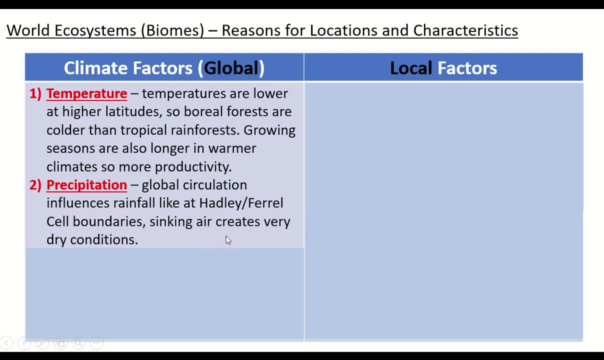 sinking air at the poles, which create very dry conditions, and you've got the sinking air around sort of 30 to 40 degrees north and south of the equator, where you find your deserts, And then, lastly, the amount of sunshine. I already 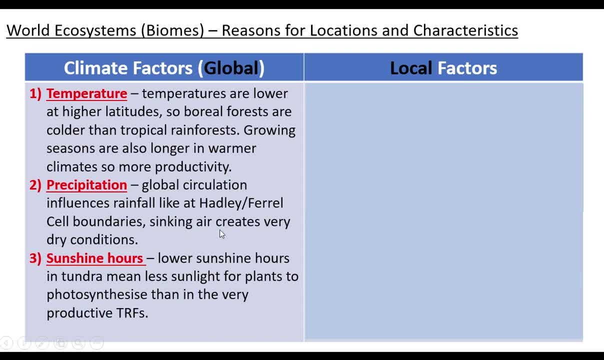 mentioned that within the temperature section, but the amount of hours of sunlight. So this relates to things like summer and winter, but you've got lower sunshine hours, the more extreme areas, so the north and south of the of the world, and that lower sunshine hours and sometimes for. 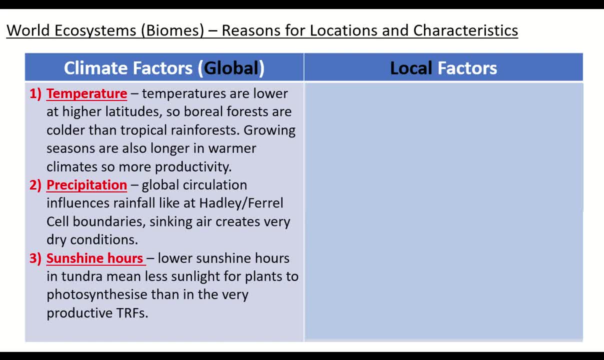 example, you know, 40 to 60 days of the year. sometimes the sun doesn't even rise or set at certain times of year. So as a result of those reduced sunshine hours, it means that you're not going to have as much sunlight for plants to photosynthesize, whereas in the rainforests they 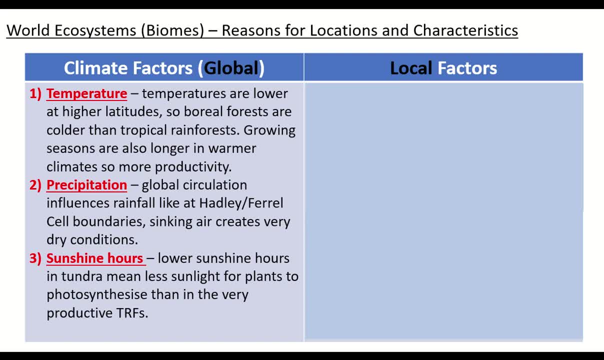 sunlight very consistently every single day and that helps those plants have a stable environment. So the local factors which can affect their sort of characteristics. these tend to be more to do with soils, The rock type, so the geology, and again this ties in with the 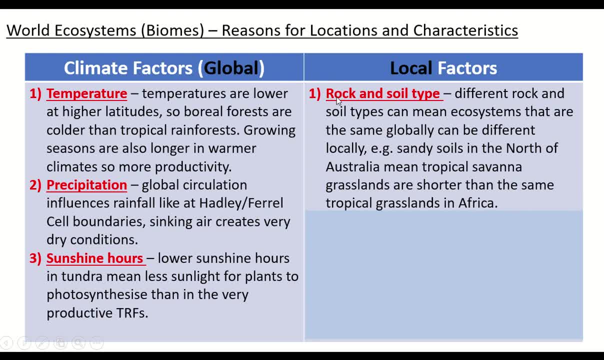 first topic from this particular paper. So if the rock type, for example, is a particularly hardy sedimentary rock, then that will determine the kind of nutrients or the mineral composition of the soils that go into it. So different rock and soil types mean that ecosystems can actually be. 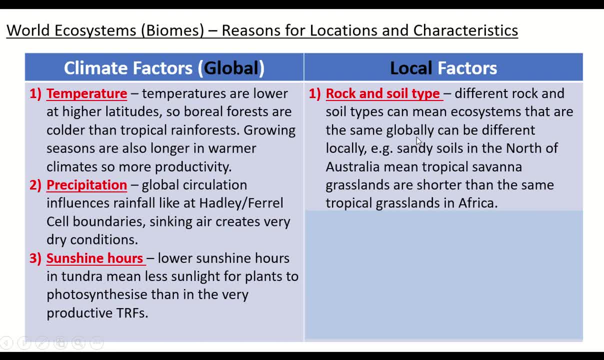 found in very similar places but be very different locally. So, for example, if you took the rainforest, if one patch of rainforest was above sandstone and another patch of rainforest was above limestone, you would find very, very different types of soil, because soil is mainly composed of the rock, that's 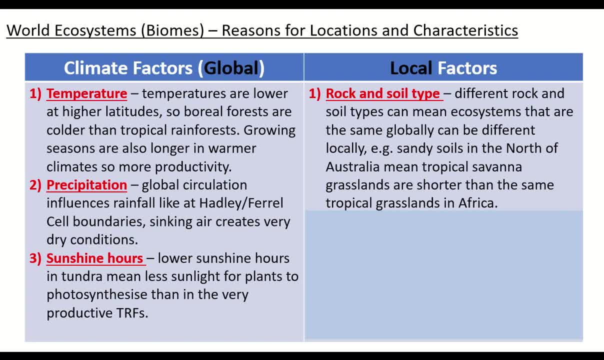 underneath it. The other thing that affects the soil obviously is the vegetation that goes into it from above. That's a picture of the soil as a whole If you took the rainforest and. But those two factors- really the rock type, which affects the soil type- mean that you can have different. 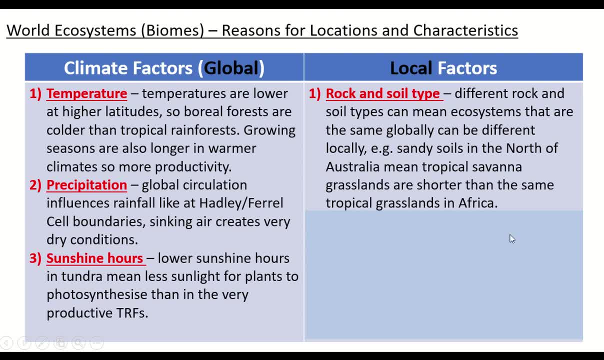 types of environment, even if it's in the same biome. sandy soils, for example, in the north of Australia, means you get tropical savannah grasslands, but they are different savannah grasslands than you'd find in Africa, which has a different soil type. and then, lastly, another 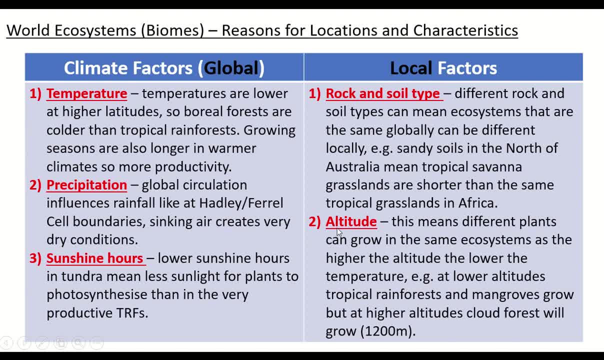 local factor is how high or low you are to sea level, so altitude. so some plants, for example, can grow very, very well at higher altitudes, but generally speaking not so many. so if you've got a very mountainous area you'll tend to find that you have fewer species. so at lower altitudes it's. 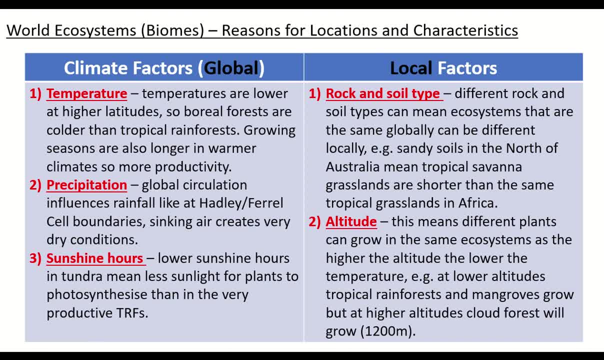 the opposite. you've got generally kind of favourable conditions for lots of plant life. that's why you'll find that tropical rainforests or mangroves, which are very productive, they'll tend to grow at lower altitudes- sorry, at lower altitudes- and then you'll find that you can. 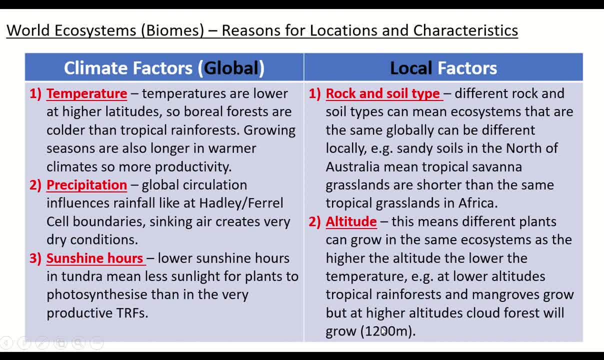 tropical rainforests grow at lower altitudes. mangroves, however, grow at higher altitudes, and cloud forests you might find them, for example, sort of 1200 meters, but again altitude, rock and soil type. these can change local characteristics, whereas where you find them, mainly globally. 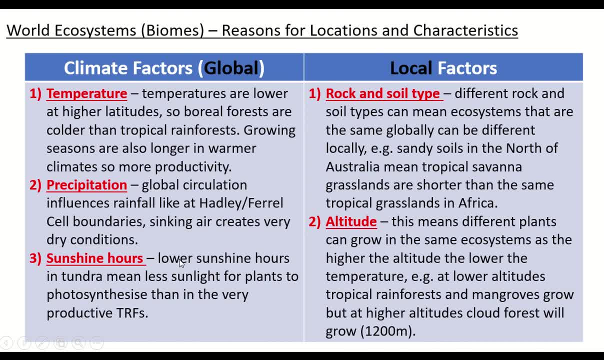 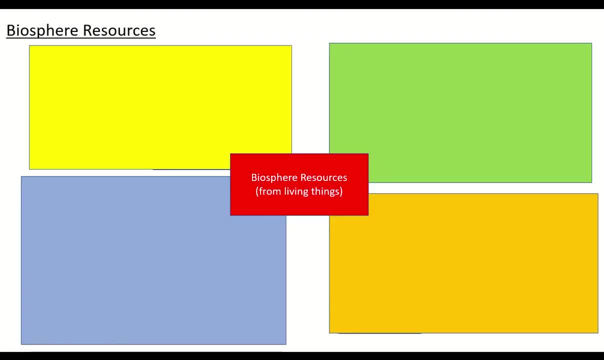 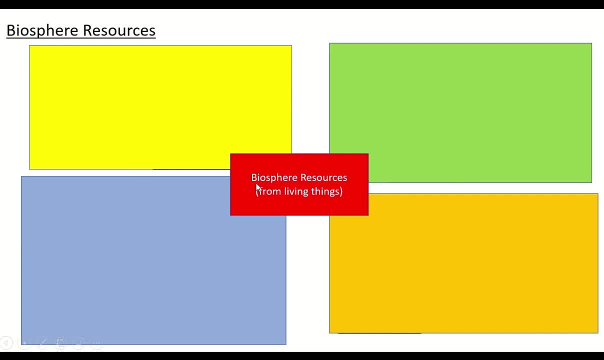 circle um. the biosphere just means um all living things, bio on earth. so the biosphere is every living thing, whether it's in the sea, whether it's in the sky, whether it's in the trees, whether it's in the, the plants, the animals and every living thing on earth. we're looking at the resources. 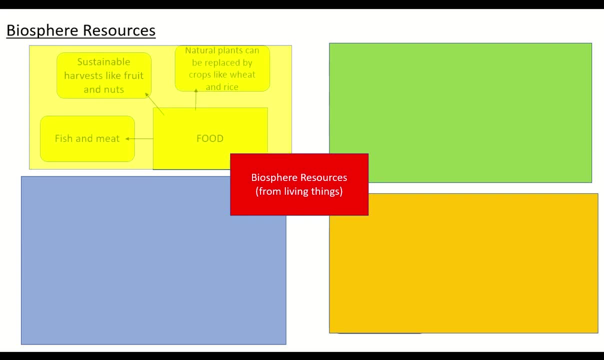 we get from those living things. so biosphere resources can include things like foods. all right, so we- we obviously eat fish, we eat meat. they are living things. they are. they provide us with a resource. they're a biosphere resource. um um, fruits and nuts- again, we also eat those- and natural plants- things like crops, wheat and rice. 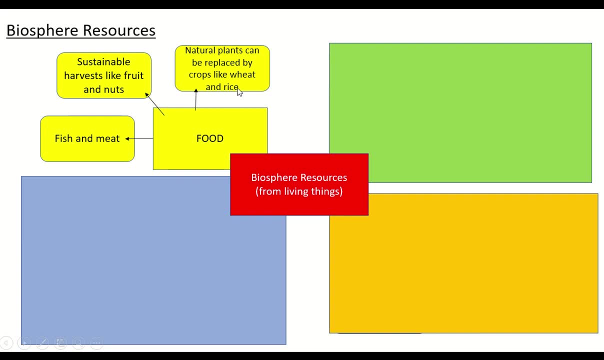 um, that we've found and then we've, we've cultivated and grown because we we use it quite a lot for lots of our staple kind of ingredients. so food is one way that the living kind of parts of the earth, the biosphere, can provide us with a resource. another way is fuel, so animal dung could be dried. 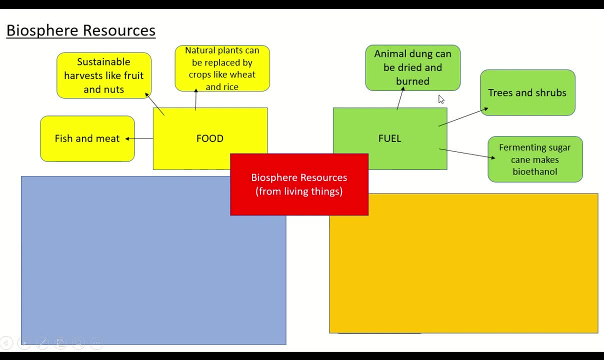 and burned, and they used to do that back in the old days, believe it or not, before I was born. obviously, trees and shrubs obviously can provide fuel as well in terms of biofuel, and if you ferment sugar cane it can make bioethanol. other areas that the biosphere helps us is through medicine, so a lot of 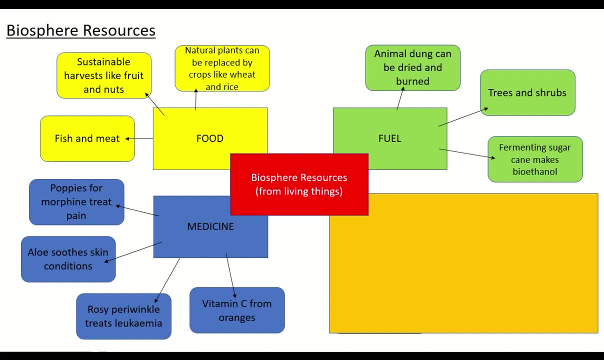 the rainforests provide us with lots of medicines that we use still today. so, but even more simply than that, poppies have, or the opium poppies have, morphine, which helps treat pain. back in Sherlock, the skin conditions, and again, we still use that in lots of products that are used for skin today. 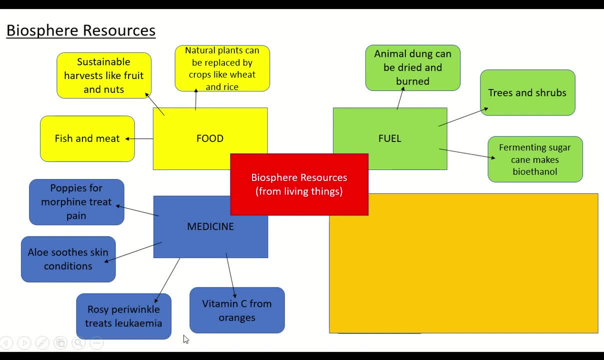 um, something called the rosy periwinkle is a plant that you'd find in the rainforest which actually helps treat leukemia, which is sort of brain cancer, and even just something as simple as vitamin C from oranges is really really good for for us as humans in terms of medicine and then, lastly, building. 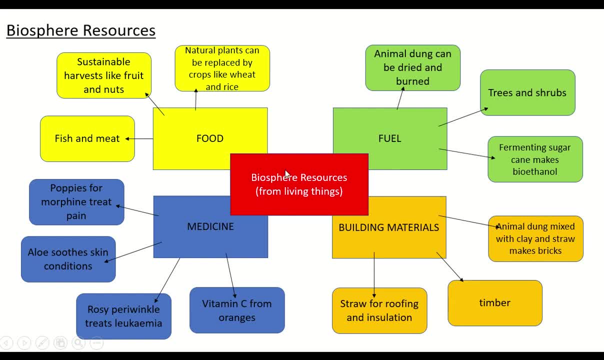 materials. so other ways that the living system or living sphere provides us with things is through um animal dung again, good old animal dung. rather than just being just used for fuel, we mix it with clay and straw to make bricks for houses again. we don't do that so much now, but that was very. 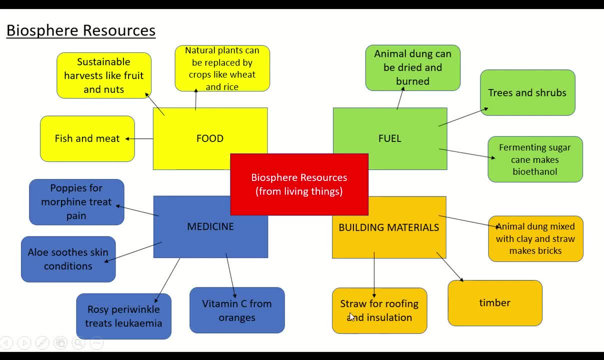 much something we used to do in in um in back in the day, and things like straw for roofing and insulation, and if you go to parts of the broads, they use things like reeds for their thatched roofs as well. okay, so these are all ways that the biosphere can provide us with lots of resources. 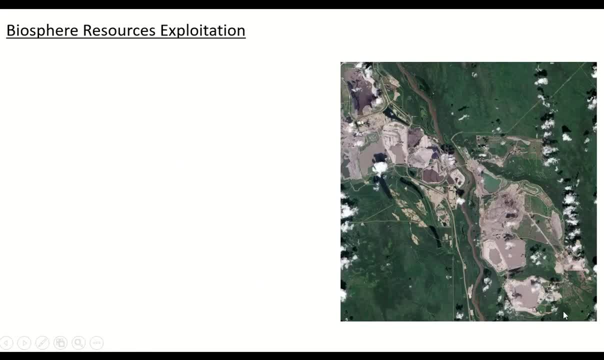 okay now, because the biosphere provides us lots of resources. okay now, because the biosphere provides us lots of resources, we use it a lot and we exploit these resources, and often this word exploitation is not really associated with being a good thing, and that's because we tend to over exploit these resources. 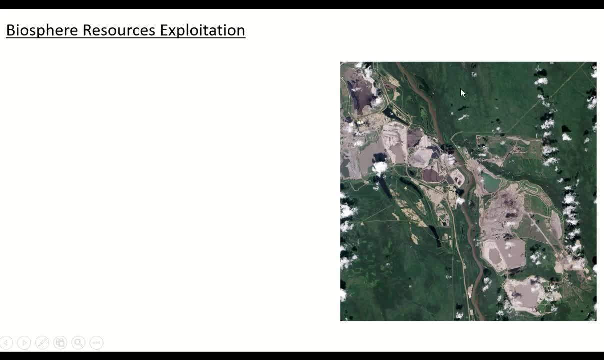 so if you look at the image on the right here, this shows you an area which has been ravaged by us exploiting the natural resources that lie underneath the vegetation. so all these brown patches here are all areas that have been deforested in order for us to access the resources. 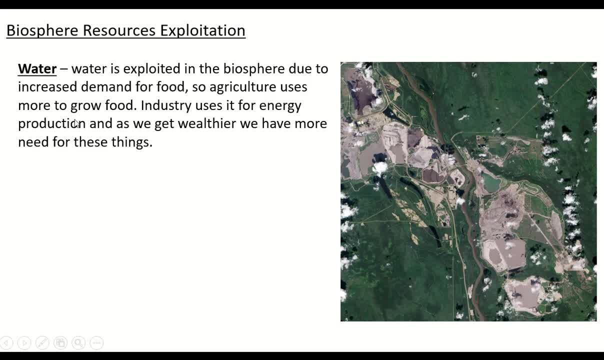 below so. foreign food, industry for making energy and obviously all the living things that live in water are affected by how much there is or isn't available to us. so we exploit the water in the biosphere. due to increased demand for food, agriculture uses it to grow more food and industry use it for energy. 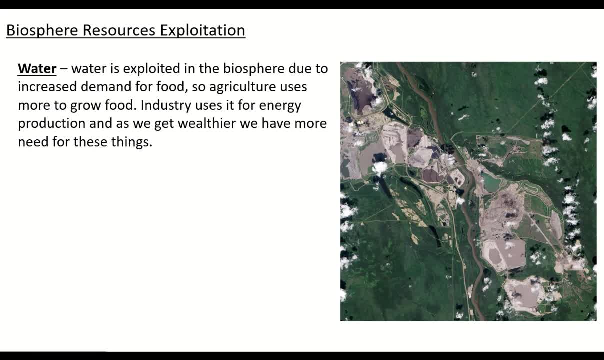 The wealth that we get, the more we have. the more stuff we have that needs energy, the more food we want to buy And therefore the more water we take out of the hydrosphere, which then links to all the living things that rely on that water. 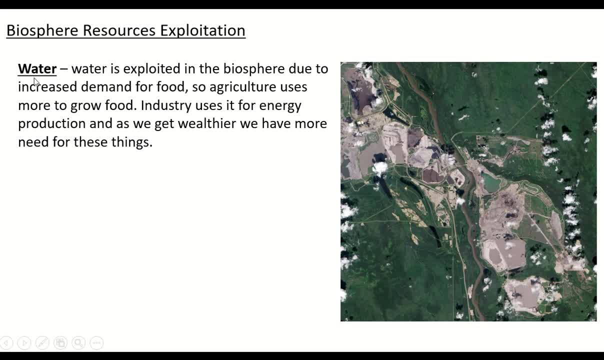 So, for example, plants and animals, they need water, just like we do, But we tend to be the greediest one of all Energy. So energy is another thing, or another consequence really, of us exploiting the biosphere. So biofuels mean that we've got again less space for growing crops for food or for natural vegetation. 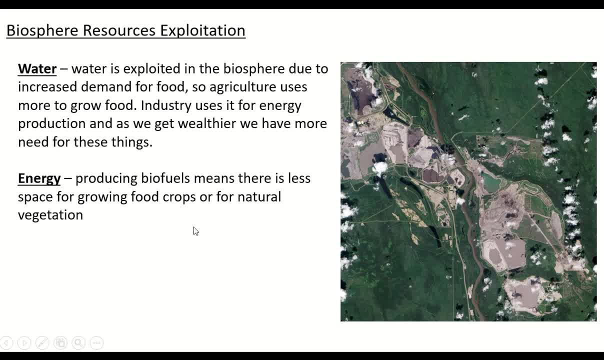 But again, our thirst for energy is all consuming and all quenching And we need more energy, as much energy as we can provide really for our growing wealth and all our stuff and our gadgets, And then, lastly, we also mine. 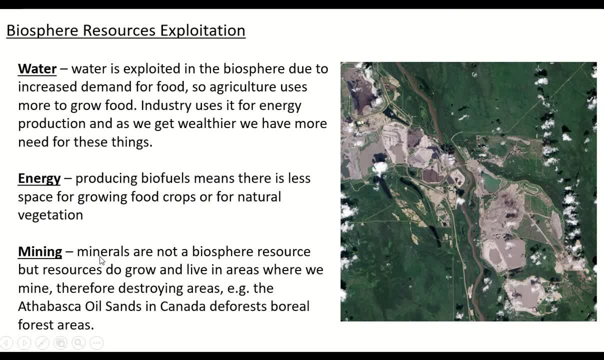 And this is not a biosphere resource- minerals- but because the minerals tend to be underneath things like rainforests, we get rid of those areas in order to get the minerals. Now, one of the most Valuable minerals to us as humans is oil, and oil is a former living thing. but the Athabasca oil sands in Canada are deforesting massive areas of boreal forest. 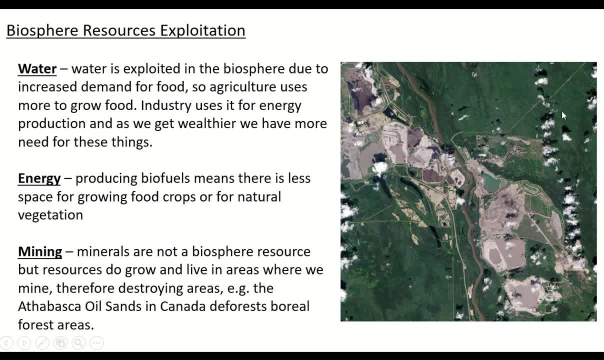 And that's what you can see here. This is the Athabasca tar sands- or sorry oil sands- of Canada, where we've stripped away the trees and we put these big kind of lakes and pools in for purifying and all sorts of stuff. 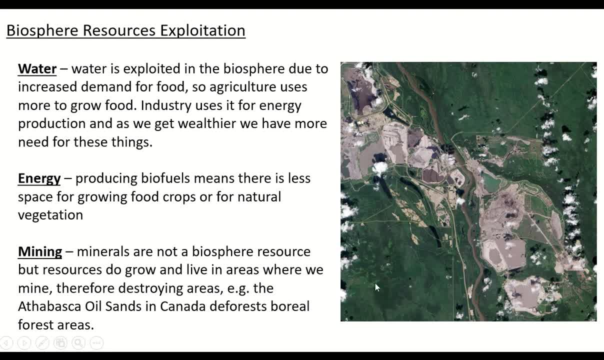 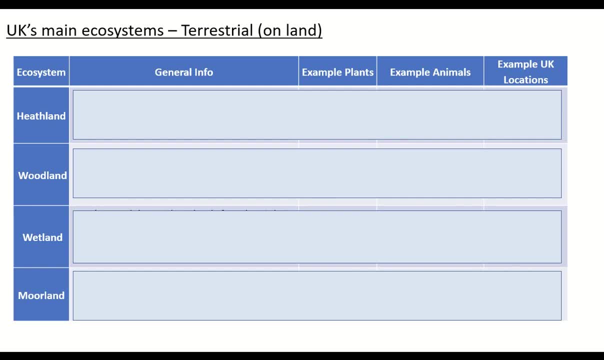 And it just leaves this big scar on the landscape and destroys all these animals habitats. So now going more locally, so let's look at the UK's ecosystems, because the first section. now we've looked at world ecosystems, world biomes and how we exploit them for the resources they provide us. 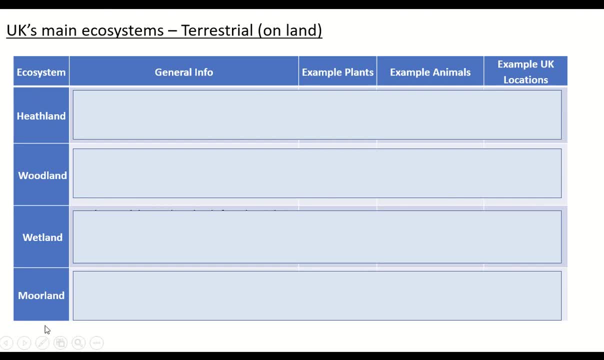 Now, closer to home, we've kind of got four main ecosystems. We've got lots more than that, to be honest with you, But these four main ecosystems that the example would highlight in the in the book One is Heathland And with regards to Heathland, we've got quite a lot. 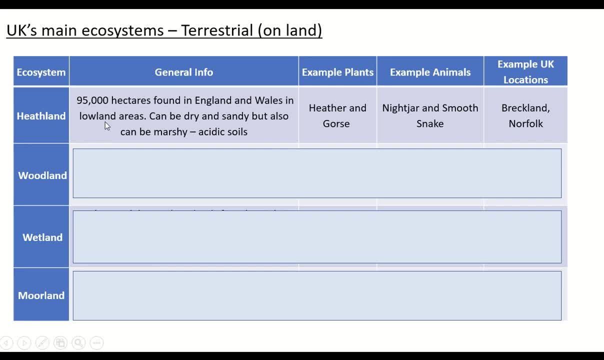 Actually in England and Wales, mainly in lowland areas- there's a bit of Heathland and west of Norfolk, for example- and they tend to be dry or sandy. They can be marshy, but the soils tend to be quite acidic. 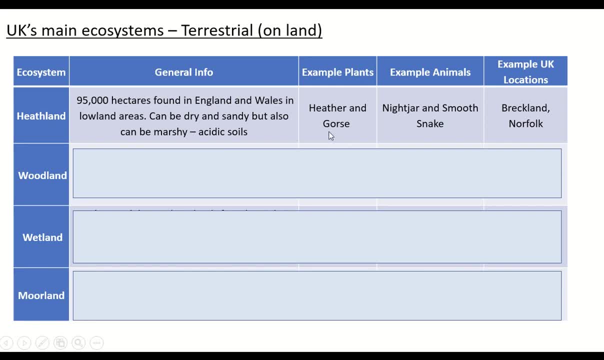 You'd kind of find heather, because it's quite hardy and gorse that very spiky plant with the yellow flowers found there. Animals that live there, species that live there- are things like the nightjar and the- excuse me- the smooth snake, which is a very rare snake in England. 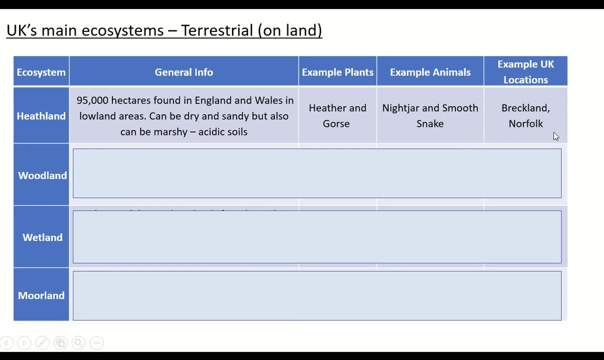 And one example of location that's near to you is Breckland in Norfolk, So think sort of Thetford Forest area. So Heathland is one UK ecosystem. We've got quite a few woodlands in the UK as well, but not all of them are natural. 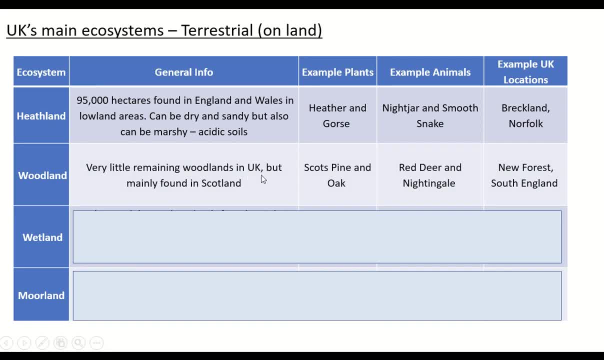 So there's very little remaining woodland in the UK compared to what it was. Imagine a time when the UK was about 80 to 90 percent woodland. This was a sort of just the scene about three or four hundred years ago. We tended to get rid of quite a lot of that. 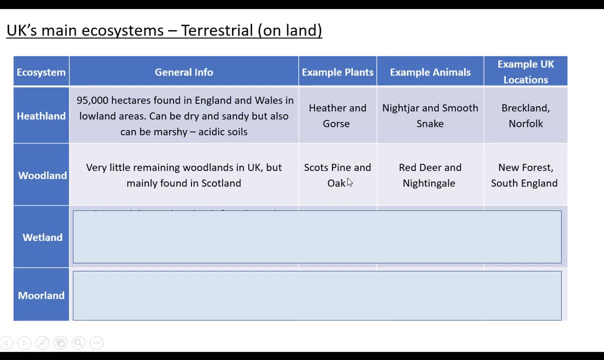 Oak is one classic example. It's a good example of a deciduous tree. but if you go to Scotland, they naturally had things like Scots pine growing. Example animals: red deer, nightingale, any species really. if you've ever been for a walk in the woods and seen these, they are good examples to use. 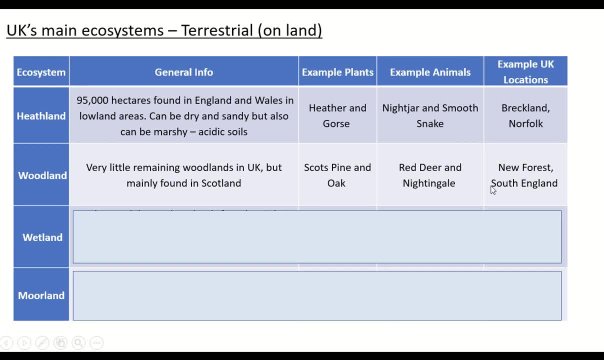 And one example we use- and I've highlighted this one because it's our case study later- is the New Forest, which is in the south of England Now wetland areas. we're really fortunate We live near the Norfolk broad. 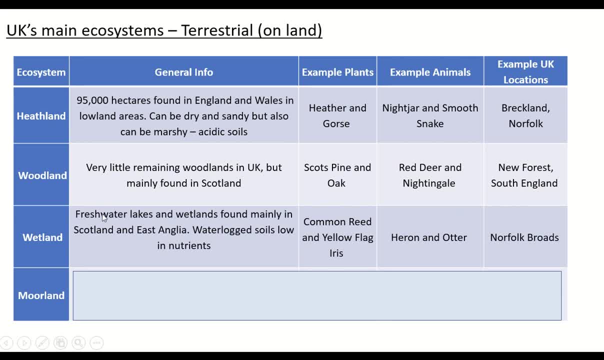 So again we've got another nice example we can just use easily, And they are freshwater lakes and wetlands that are mainly found in Scotland, but also East Anglia, waterlogged soils, very low in nutrients, And you'll get species like common reed or yellow flag iris. 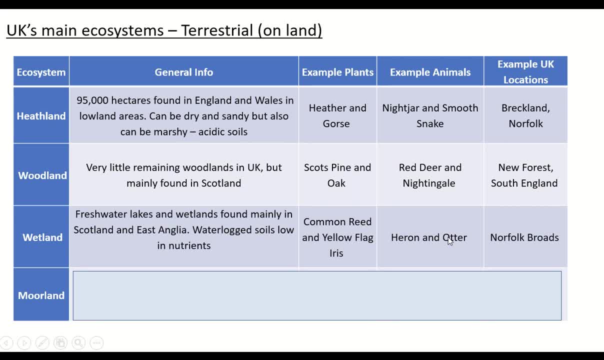 They're both sort of types of plant there, Animals, wise herons and otter- again things we associate with Norfolk quite strongly there. And then lastly moorland. Now, the difference between heathland and moorland is altitude. 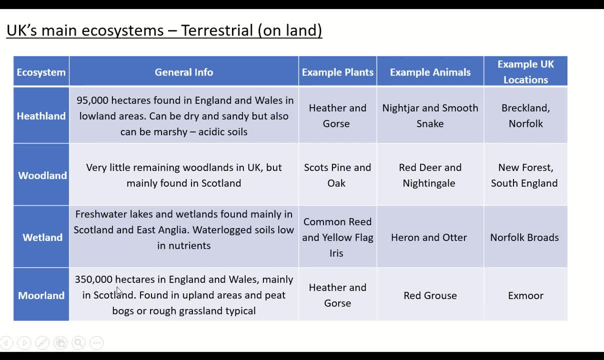 So we've got quite a lot of moorland in England and Wales. Most of it, though, you'd find in Scotland. So it's in upland areas that the soils are quite peaty, boggy, that tends to be sort of rough grassland. 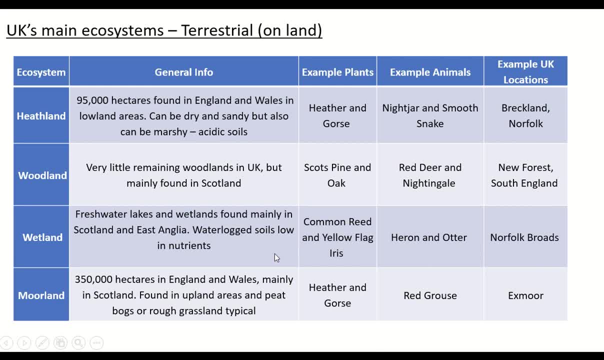 And again, just like in heathland, which is lowland areas, you'll find heather and gorse growing there, Sort of species you'd find. there are red grouse And there's an example in England of Exmoor, which is down in the southwest of England. 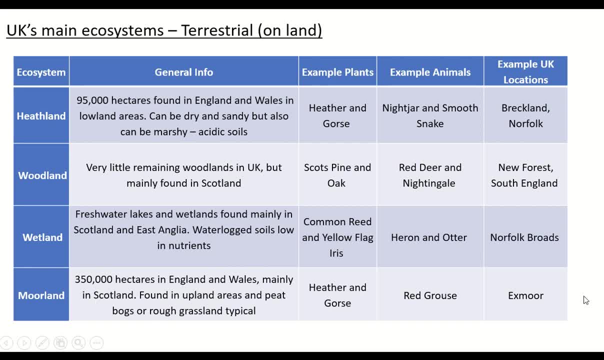 But, like I said, most of it, you'll find it in the sort of highlands of Scotland. Now, one thing that's worthwhile mentioning at this point is that there seems to be quite regular describe the distribution question for this in the exam so far. 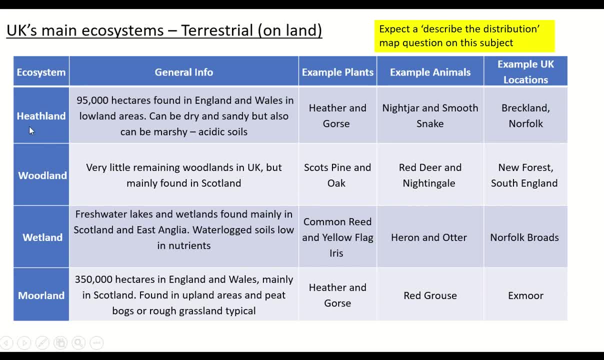 So expect maybe a map that shows potentially these areas and you maybe could describe the distribution of where you might find heathland. or, looking at the map, Where is the heathland, Where's the woodland, Where's the wetland, etc. 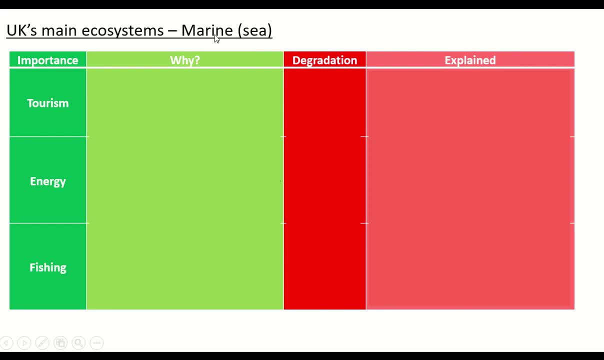 So another main ecosystem which we were looking at- going to look at separately, really, Because we kind of degrade it, unfortunately- is the marine ecosystems. We are an island, We are surrounded by sea And because we're surrounded by sea, we exploit that resource because it's very, very useful to us. 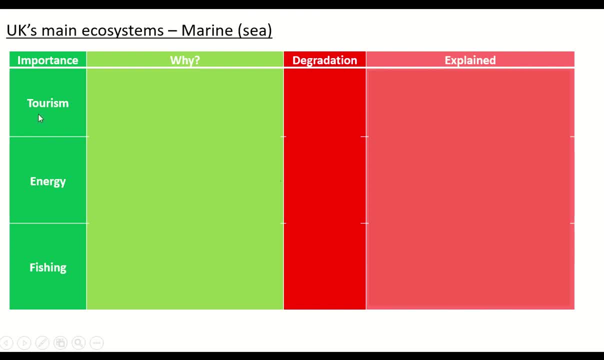 Now there are three ways in which the marine or marine environments or marine ecosystems are important to us in the UK. One is through tourism. Tourism generates loads and loads of money for us in the UK And as fishing is declined, tourism is kind of taking over. 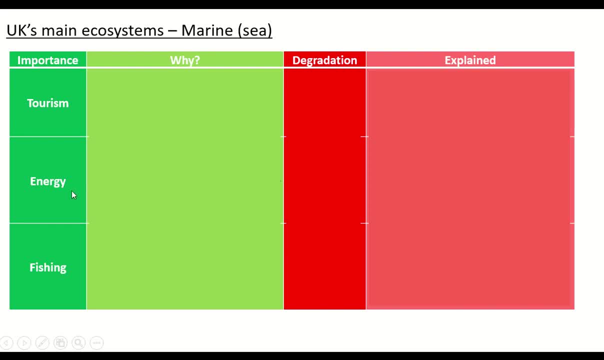 We also use it very much for Offshore wind farms. so energy, but in our North Sea deposits, not only is there the potential for wind energy, but we've got our oil and gas fields out in the North Sea, So it's an incredibly important energy resource for us. 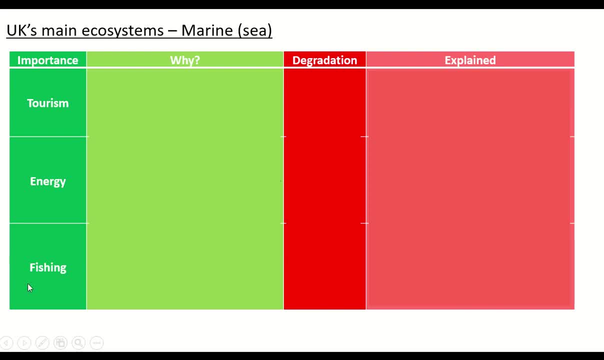 And finally, there is still fishing going on. It's not as much as it used to be, but our fishing grounds are incredibly important to a lot of people in this country. So why is tourism so important? Let's just give you some specifics. 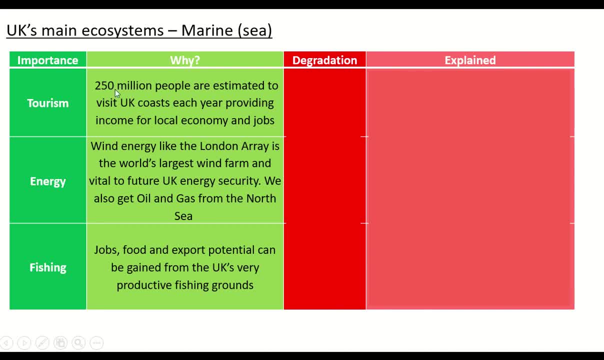 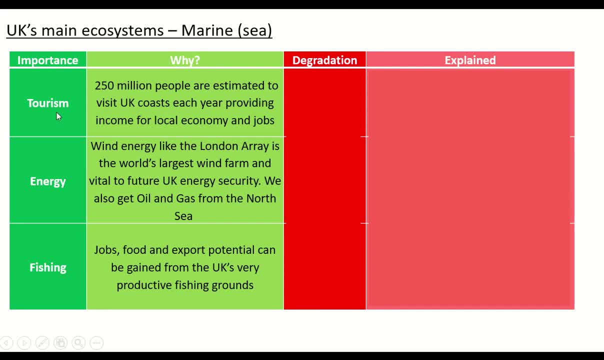 It doesn't mean there's necessarily swimming in the sea, but they do like to be beside the seaside. Now. that provides lots of jobs and money for the locals, which is invaluable to us, really. With regards to energy, the London Array, which you'll talk a bit more about in topic three of paper two, which is the world's largest wind farm, although that will change all the time. 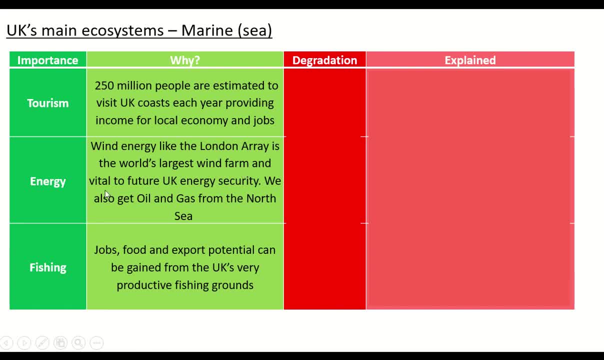 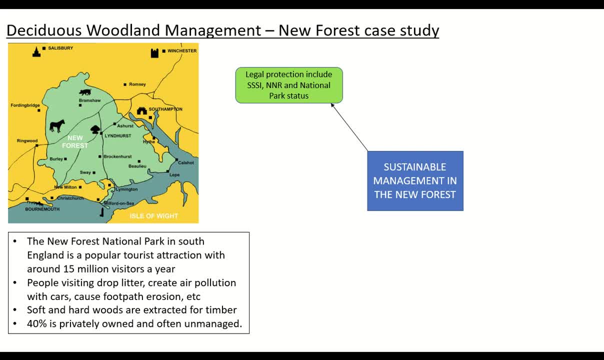 Yes, there's not as many as there were, but still quite a few jobs in fishing. the new forest is a national park, which means you cannot do certain things there. it's very restrictive. it's also got within it several sites of special scientific interest, or sssis. 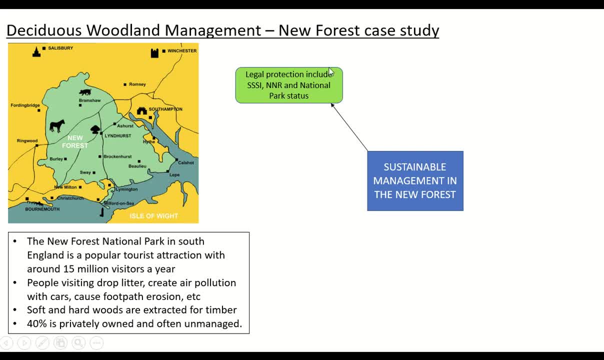 and national nature reserves as well. so there's lots of legal protection around that and with all the sites that occur in the new forest also. they've introduced a replanting scheme where, rather than replacing conifer deciduous trees with conifer trees, they actually replace deciduous 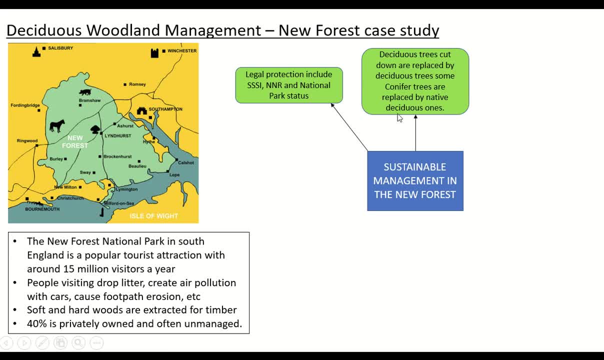 trees, with deciduous trees, which is the way it should be. they are slower growing, but also they are more native species, so it's important that we do that. they also allow certain places to become honeypot sites. now, what that means is: let's take an example, let's pretend, let's say I'm not sure. 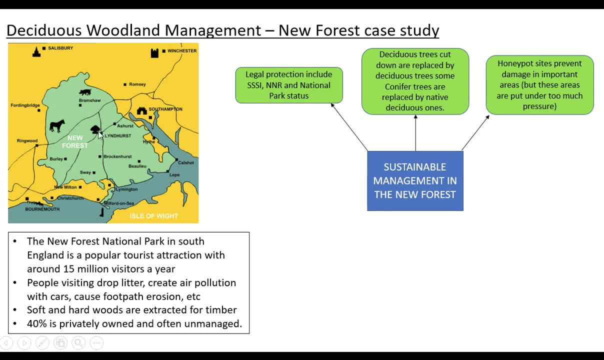 if this is the case. but let's say Lindhurst was really popular honeypot site, a place where there's lots of car parks, there's still nice woodland there and some wild horses etc. but if you attract most people to go to this area, it means that places maybe like bramshaw and burley and sway and brockenhurst and 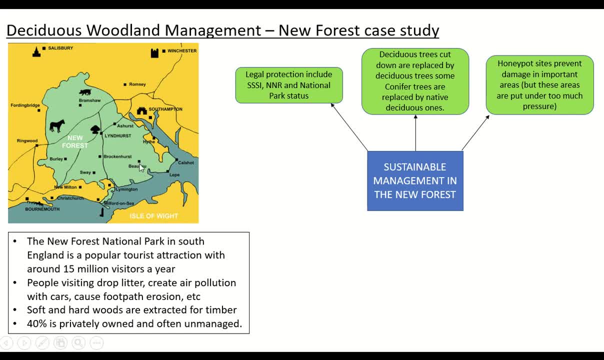 bolew or wherever that is. um, they are more protected because everyone's flocking to this place, because it's easy to park, there's a mcdonald's near there or you know, whatever it might be. so a honeypot site means that you maybe sacrifice this area a little bit and it's a bit. 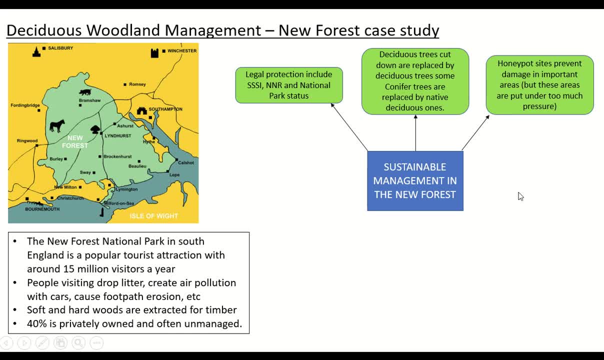 damaged to help protect all these other areas around it. um, but often that can mean that this area becomes under too much pressure, which isn't always the best thing and the locals not so keen on that. um, if i used a norfolk broads case study example, think roxham. you go to roxham. 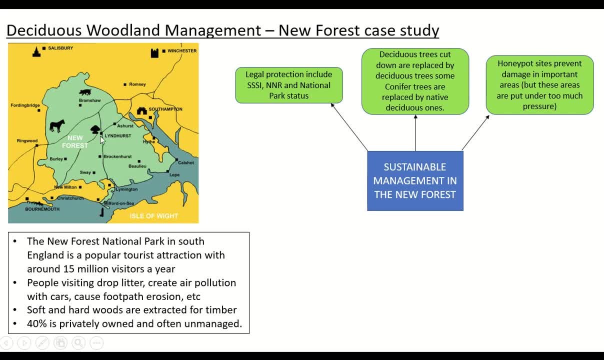 go to roy's. you've got all the shops there: big staid boat yard, there's a mcdonald's there and that helps protect places like ramworth uh, which uh have. they're more of a nature reserve. feel to them very quiet, very little traffic, small little car park um to discourage as many people from. 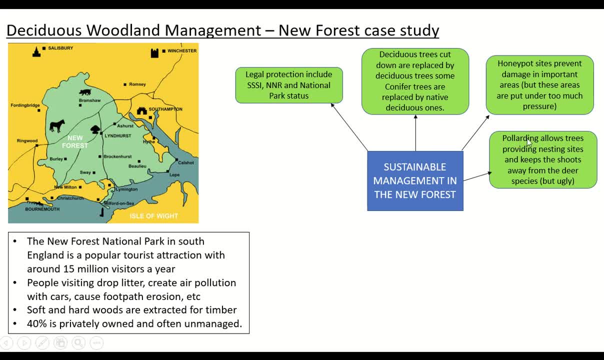 going there. um, in terms of, uh, tree management specifically, they can use pollarding. now, pollarding is where you essentially chop back the branches and then they'll keep shooting new branches, because a lot of trees are very resilient, and that's great, because what it does is it provides nesting sites for birds, but it also 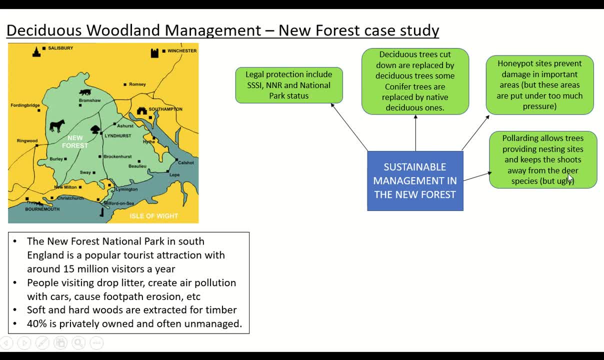 keeps any new shoots away from deer, because deer are a real pest in this country. deer could be. it could do with being shot a few more times and eaten by us. if you see venison, the butchers go and buy it because there's more market for it. it means they'll shoot more deer. 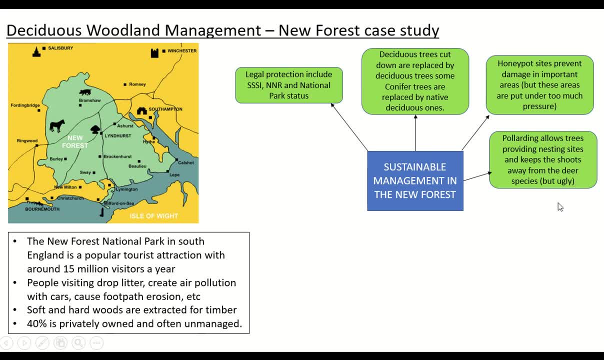 deer kill our trees. there's no natural predator in the uk for deer and so, um, they pollard to try and stop the deer nibbling at the kind of the new shoots because they're far too high for the deer to reach. but unfortunately pollarding is a bit weird looking. it makes the tree look a bit ugly.